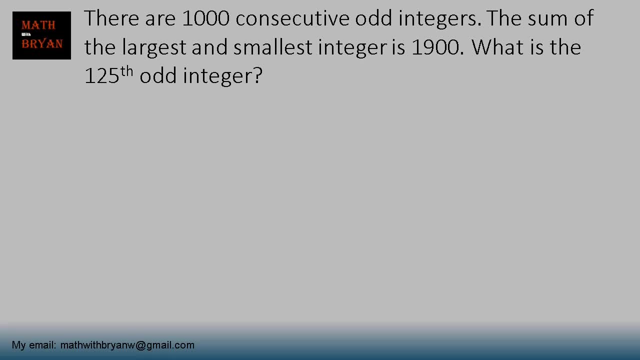 times an integer. so the general form of an even integer n can be expressed as: n equals 2k, where k is an integer. So what does it mean when we say that an integer is odd? Well, it means that it's one less or one more than an even number. 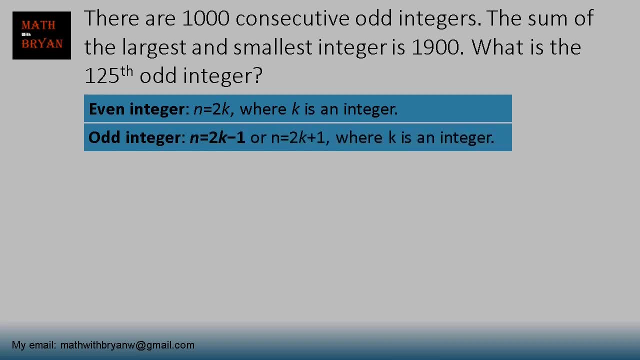 Therefore, the general form of an odd integer n can be expressed as: n equals 2k minus 1 or n equals 2k plus 1, where k is an integer. Suppose the first or smallest odd integer, n1, equals 2k minus 1.. The second odd integer, n2, can be written as: 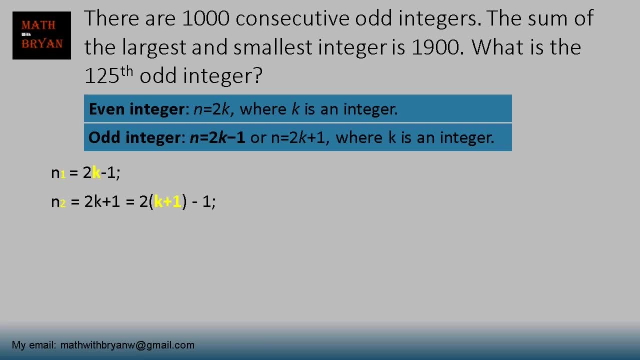 2k plus 1,, which is equal to 2 times the sum of k and 1 minus 1.. The third odd integer equals to 2k plus 3,, which can be written as 2 times the sum of k and 2 minus 1.. And the fourth odd integer: 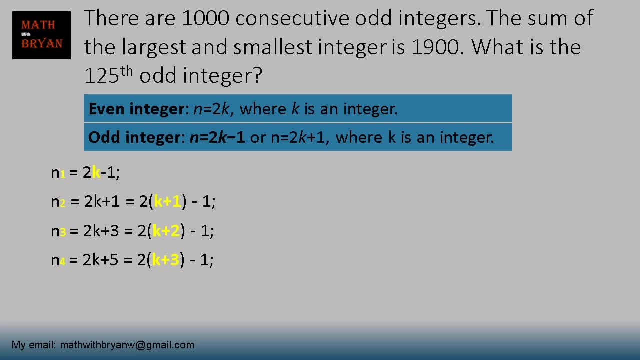 can be written as 2 times the sum of k and 3 minus 1.. Following this rule, it is easy to write down any number among the 1000 consecutive odd integers. Obviously, the smallest integer and the largest integer is n1 and n1000, respectively. We can use this formula we got on the left, then combine: 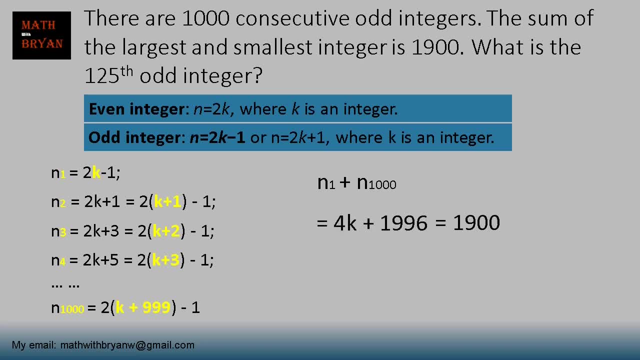 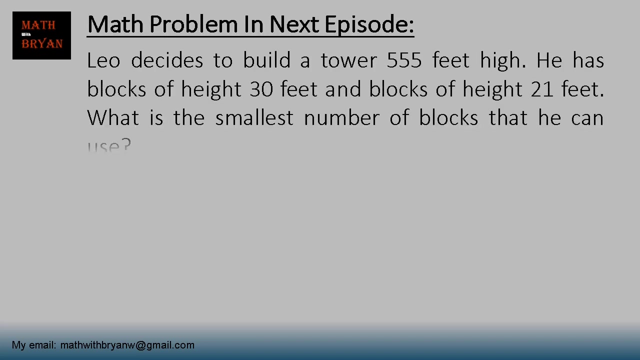 like terms to get 4k plus 1996, because its sum is 1900,. so we can simplify to get: k equals negative 24.. Substitute into our formula n125.. The result 199 is our answer, Our math problem. in the next episode, Leo decides to build a tower 555 feet high. He. 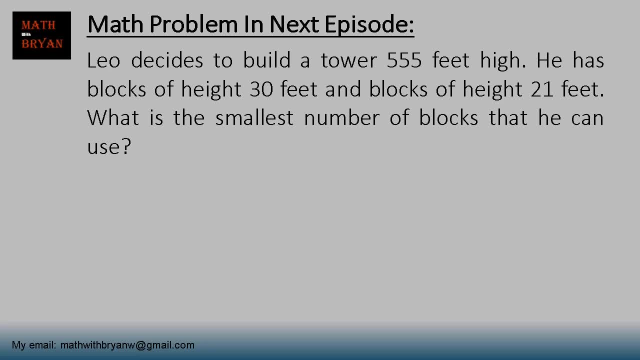 has blocks of height 30 feet and blocks of height 21 feet. What is the smallest number of blocks that he can use? That's for today. Thank you for watching my video. Please leave a like. it means a lot to me. Check out this.